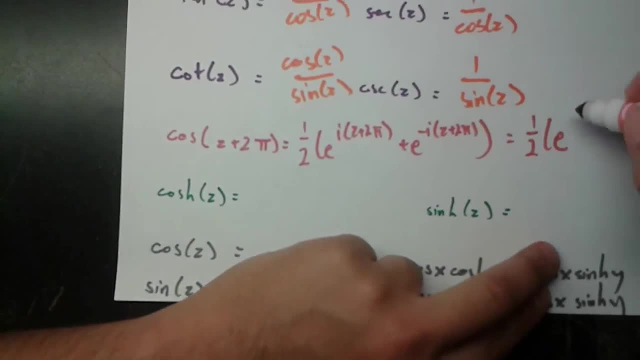 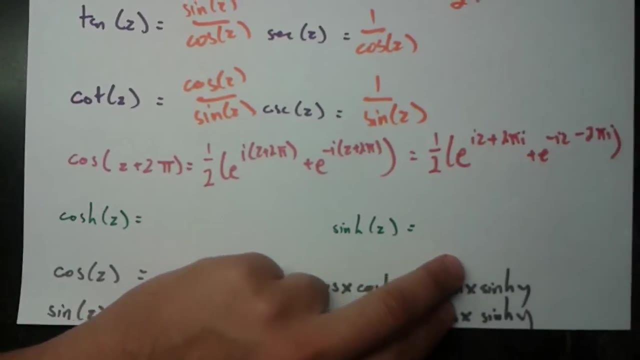 And now we're going to expand this out. We're going to get 1 half e to the i z plus 2 pi i plus e to the minus i z minus 2 pi i. Now this looks a little bit nasty, but we're just going to keep simplifying. 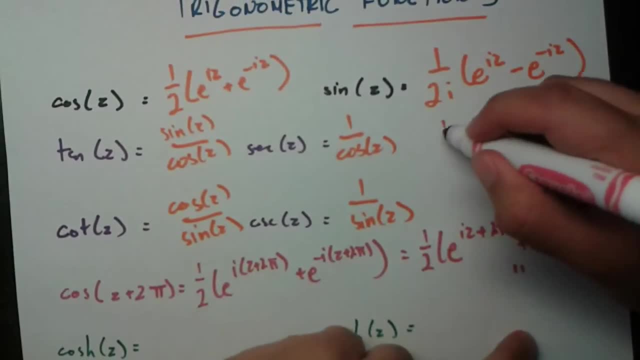 So this equals- We'll do it up here- This equals 1 half e to the i z e to the 2 pi i plus e to the minus i z e to the minus 2 pi i. And the reason I can do that is if you go back to the exponential video. 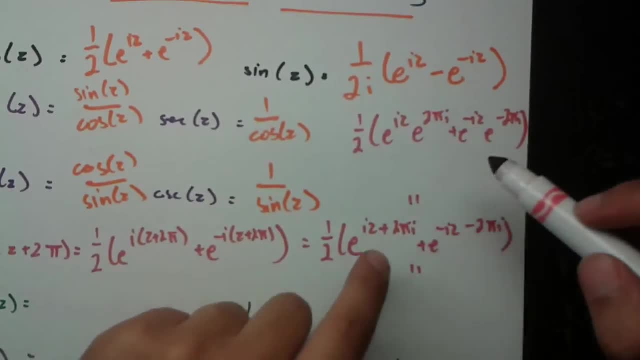 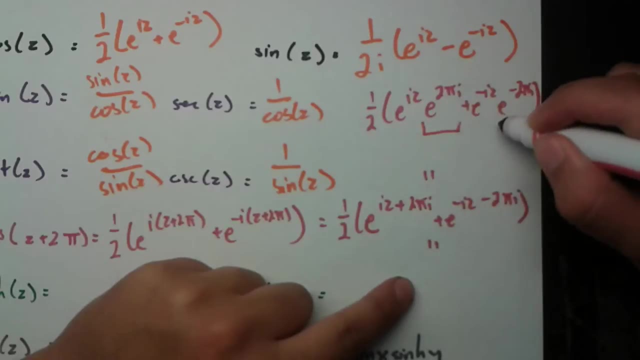 you see that, like in real numbers, when we have e to the something plus something, we can just break it up as: e to the first thing times e to the second thing. And now we need to focus on these two terms: e to the 2 pi i and e to the minus 2 pi i. 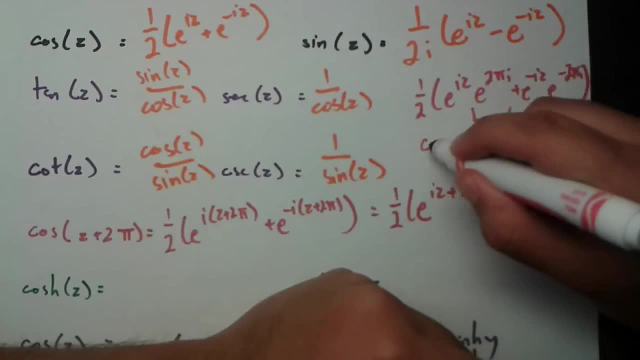 So for the first one, we see that from the exponential video this equals cosine Of 2 pi plus i sine of 2 pi, And cosine of 2 pi is 1.. And sine of 2 pi is 0. So this i term goes away. 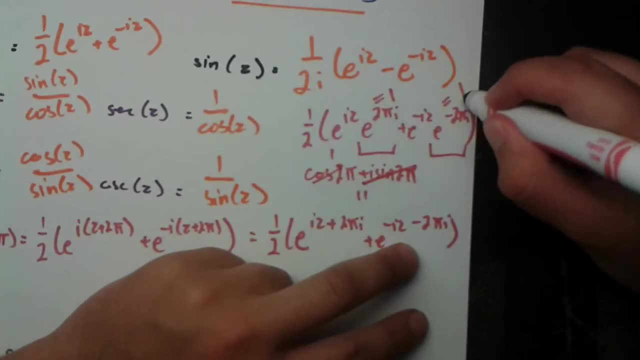 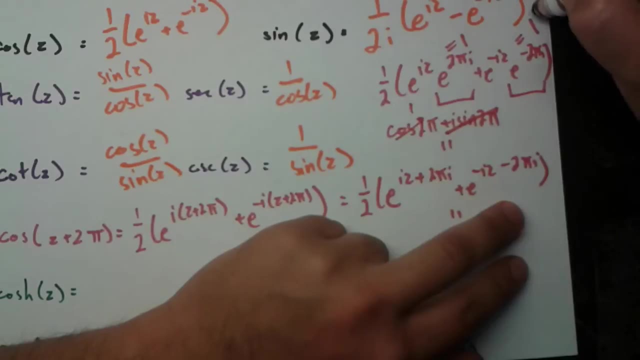 And this just equals 1.. For the same reason, e to the minus 2 pi also just equals 1.. So what's left? after all this dust clears, We see that what's left is, And I'll put it up here. 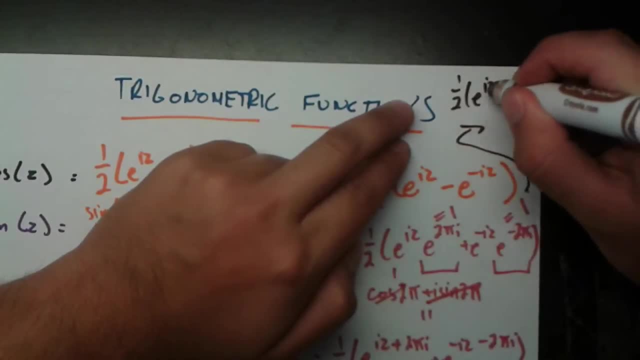 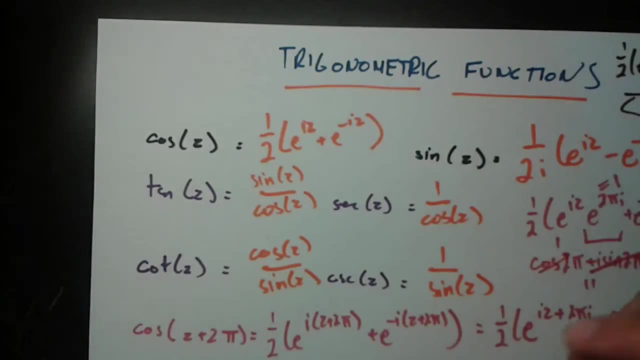 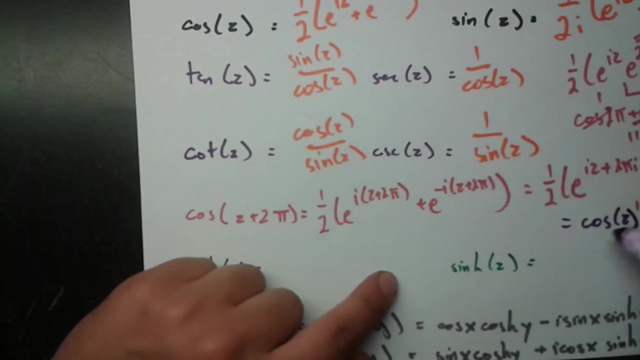 What we have left is just 1 half e to the i z plus e to the minus i z. And where have we seen this before? We see it right here. So that's. the interesting thing to note Is that cosine of z plus 2 pi is the same thing, is equal to cosine of z. 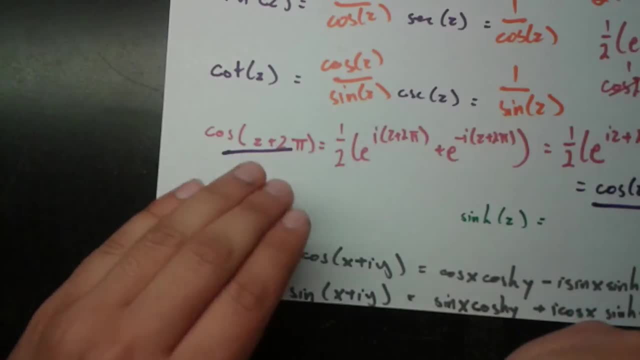 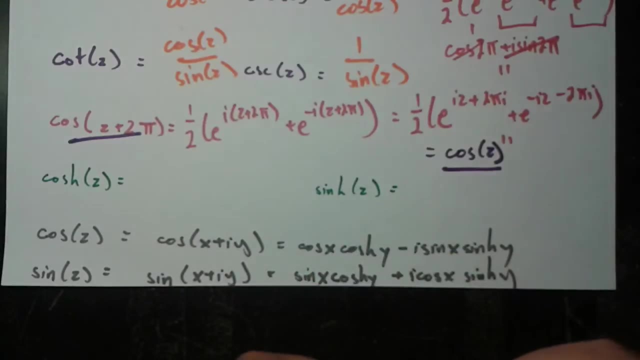 And if we do the similar calculations for sine, we'll find that sine of z plus 2 pi is also equal to sine of z. And what does that mean? That means that the period of cosine and sine, even for complex numbers, is 2 pi. 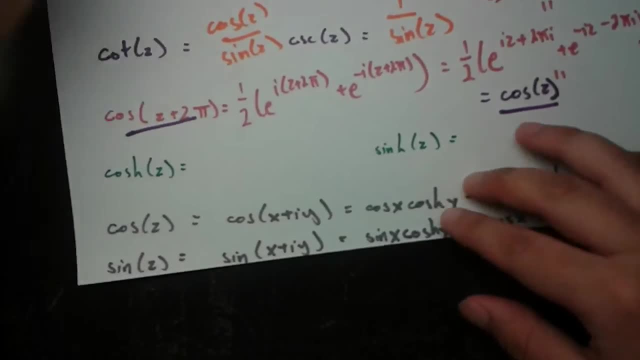 So that's a good result to keep in mind. Now we'll go on with our definitions. You might have seen my videos about Cauch and Cinch, or hyperbolic cosine, hyperbolic sine, in previous videos. But just a refresher. 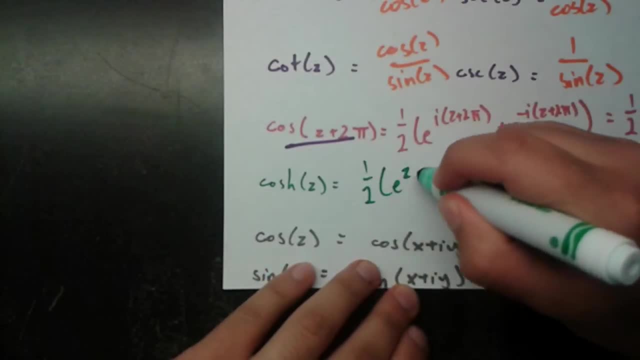 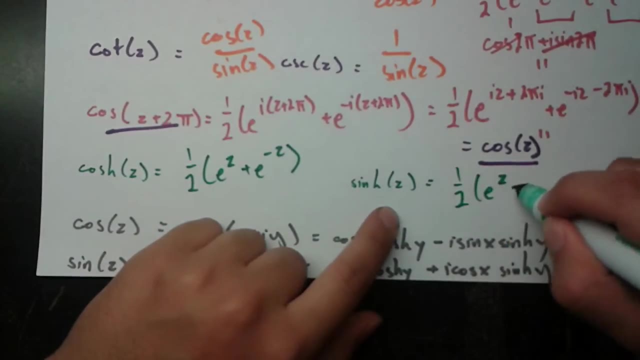 Cauch of z is defined as 1 half e to the z plus e to the minus z, And Cinch of z is defined as 1 half e to the z minus e to the minus z. Okay, And now the last thing we have to note. I've just written out already. 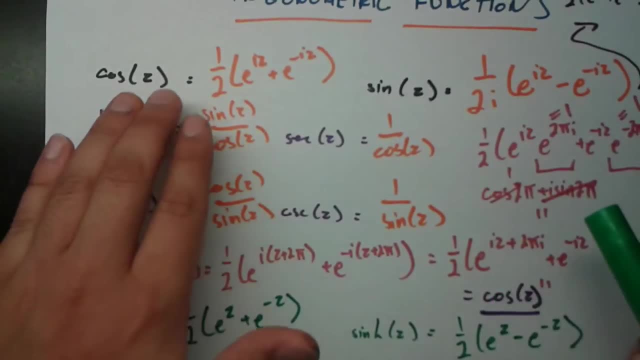 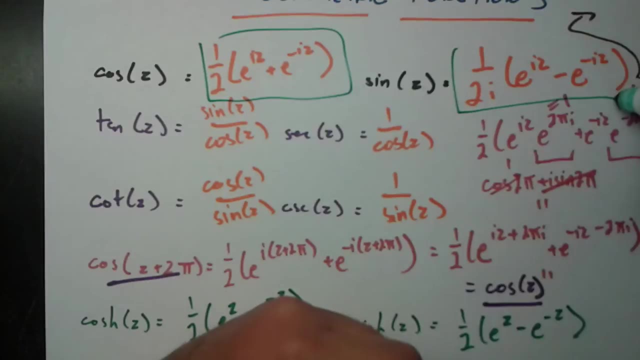 And this is a different form of cosine and sine. So we've seen this form of cosine written as like this and sine written as this definition. But the thing about these definitions is that, while they're nice and compact, you can't really tell the real and imaginary part.